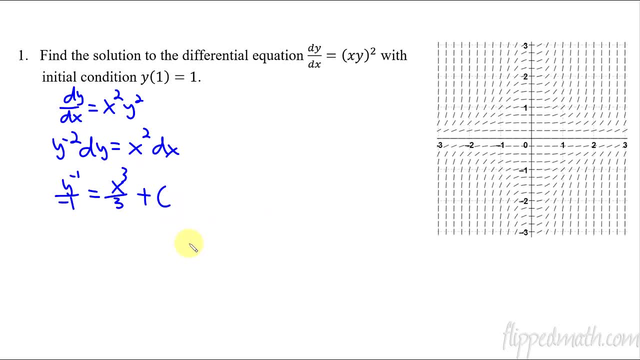 3 and then plus my unknown constant. So at this point we have a decision. we can try and figure out what this constant is right away. plug in 1 comma 1, Or you can solve for y and then figure out what the constant is. It doesn't matter what order you do it in. 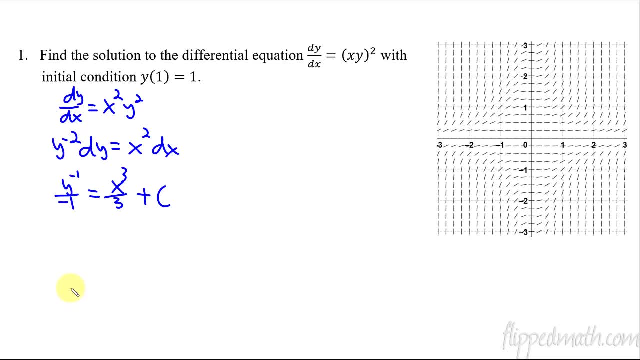 It's really up to you. Sometimes there's an easier way of doing it, but you'll get used to that. the more of these you do, Which problem might make it easier? but you'll get the same answer, So it doesn't really matter. So I'm gonna. 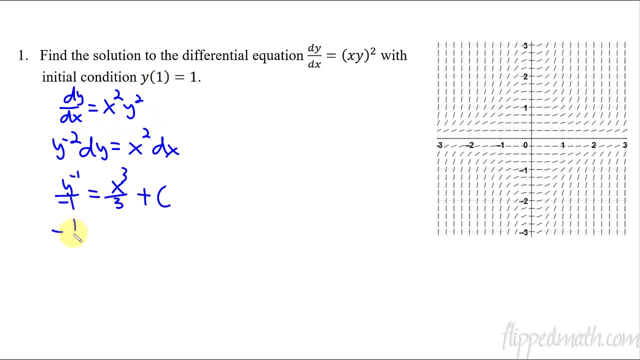 Go ahead and plug in the 1- 1 right away. So this is the same thing as negative 1 over y, which in this case was a 1. that equals 1, 3rd plus my constant C, and then subtract 1- 3rd from both sides. 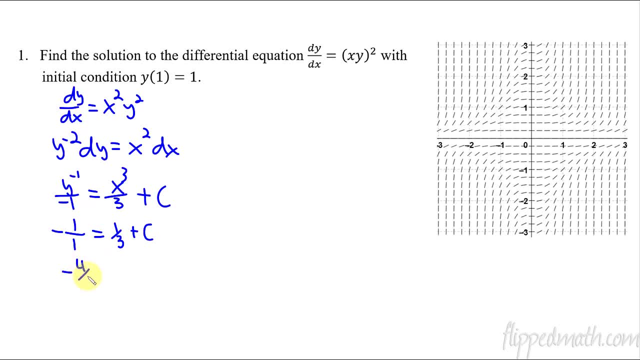 So this is negative 1 minus 1 3rd, That's negative 4 3rds. equals C. Now I know what C is. I'm going to come back up here and start over and start solving for y. So this is negative 1 over y. That's what this first part of it is. equals x. 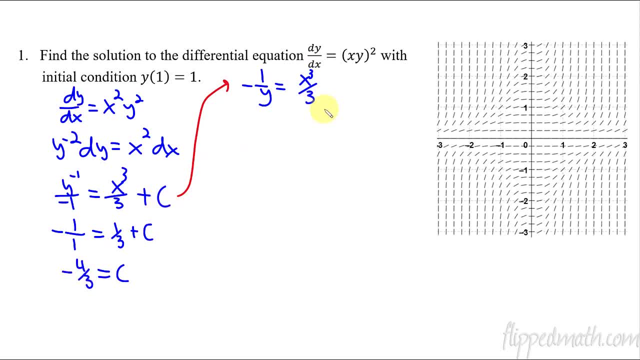 cubed over 3 and then my C is a minus 4 3rds. So I'll say minus 4 3rds. now This is nice because I have the same denominators, So I'm gonna put this all together and get rid of this negative at the same time. So this becomes 1 over y. 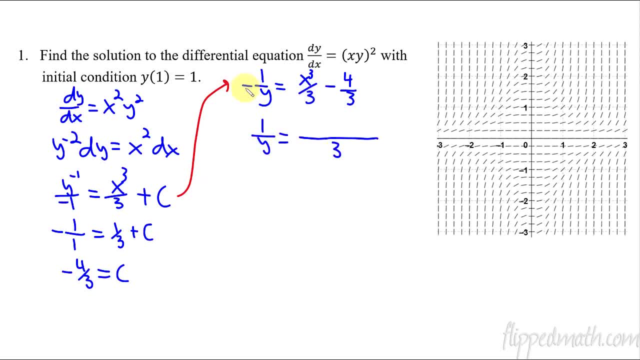 Equals, so I have all over 3, and then if I distribute this minus- because I multiplied both sides by negative- It's now negative x cubed plus 4, or I could rearrange it and say 4 minus x cubed. Okay, so I'm just doing little algebra tricks to kind of clean this up, make it look a little bit nicer. 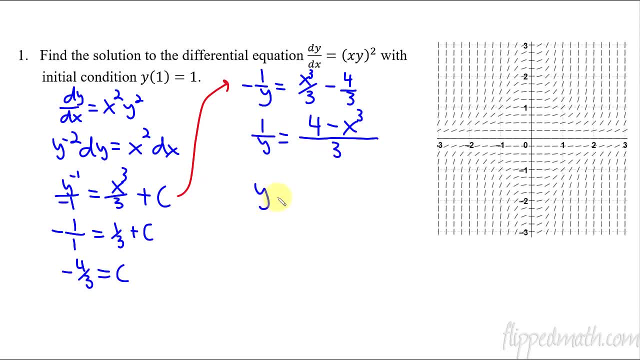 And now the reciprocal of both sides creates this: y equals, and now I have 3 on top and 4 minus x cubed on bottom. Okay, so now we go over to what does the graph look like? goes through the point 1: 1?. 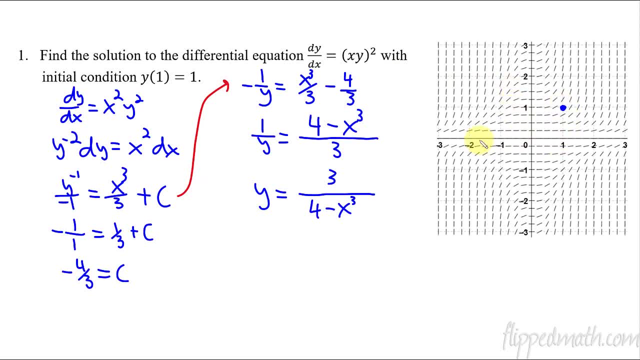 We're gonna sketch this graph, so 1: 1. now I'm only sketching the graphs. You'll have to sketch the graph on some of them, But I'm only sketching the graph for, actually, examples number 2 & 3, so you can see something weird that's going on. 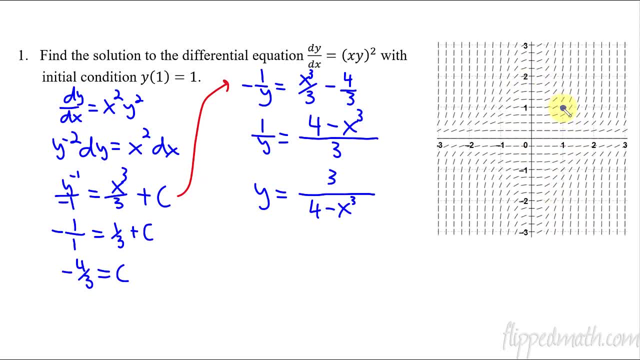 This is a really strange graph. I actually had to graph it myself to figure out what graph this is. I actually had to graph this thing to figure out what's going on And at first I thought it was like a cubic, like it was gonna do something like this. 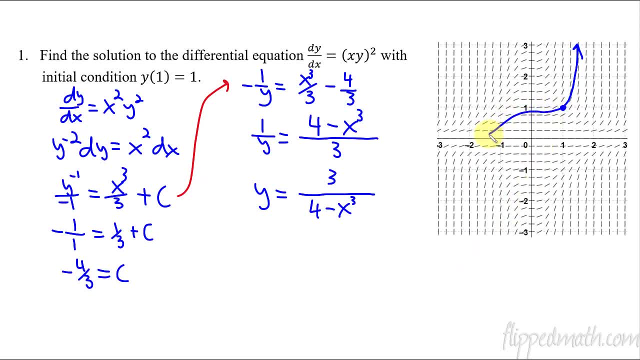 But that's not what it does. it flattens out, curves down and then it's asymptotic. It has an asymptote- Oh, that was awful. It has an asymptote right there that, as it approaches 0, if you go off to negative infinity, 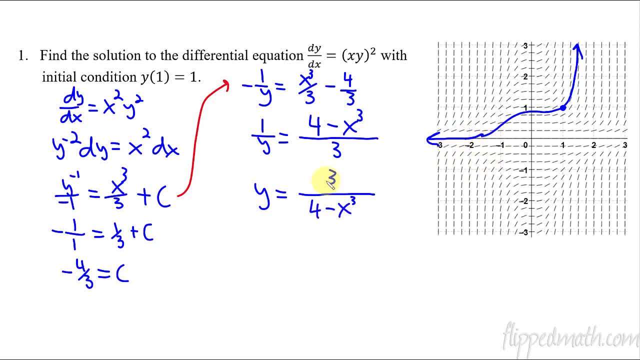 You plug a really big negative number in here. It's 4 plus infinity, So that whole fraction approaches 0. So that's what's happening with a graph. You don't stress about that. you had to know exactly what that graph was doing. There's some little tricks you can do here and there to help you figure it out. 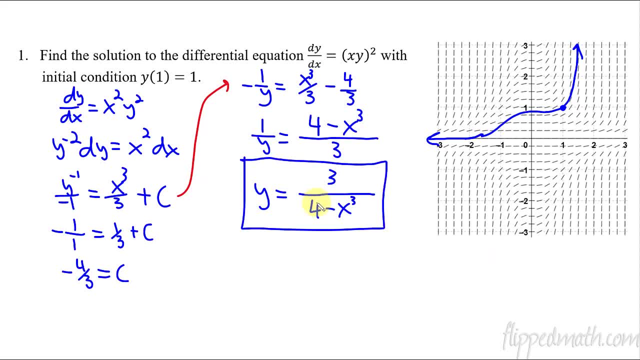 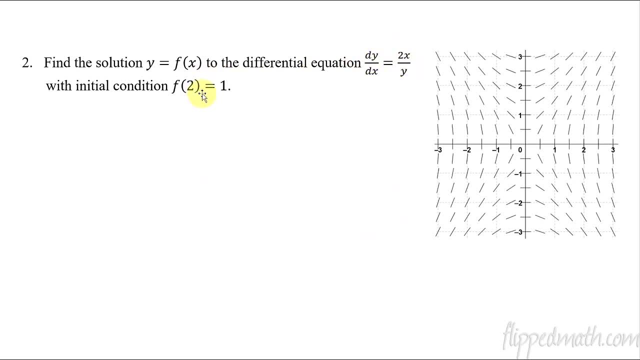 But don't worry about that one, I'll show you the graphs on the next ones. I should have blocked my answer, though That was the final answer right there. Number two: we're gonna take this differential equation, use that initial condition. So let's get started here. I'll separate the variables. 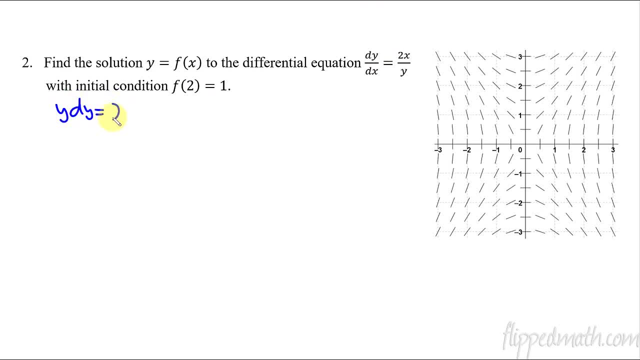 I get a Y on the left, Dy equals, and then I have my 2x DX on the right. So I'm just separating the variables here. now integrate both sides. I get y squared over 2 Equals. the 2 is gonna end up canceling. I get x squared and then plus an unknown constant. 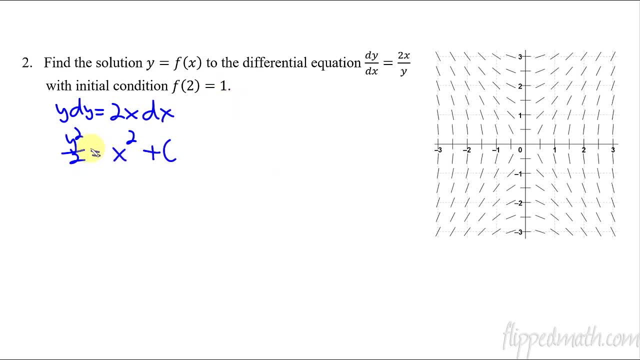 So again, this is where you could do. we want to get Y by itself. Do we want to go ahead and just plug in the 2 and 1 and figure out what this C is? I am going to actually multiply both sides by 2 so I get y squared equals 2x squared. 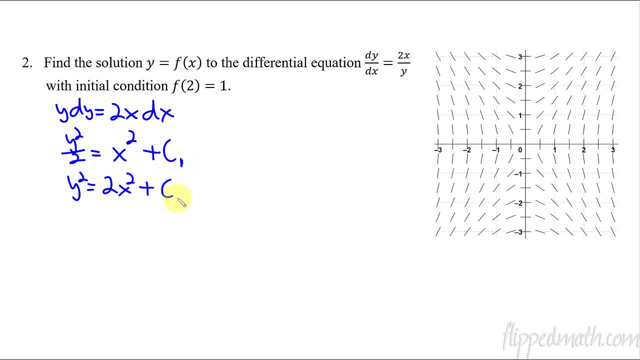 Plus, and now it's not the same constant anymore. This was a constant number 1. now It's constant 2. It's a different constant, And the reason I multiplied by 2 is for me. I think it now makes this a little bit easier to work with, since I wouldn't have a fraction if I plugged a 1. 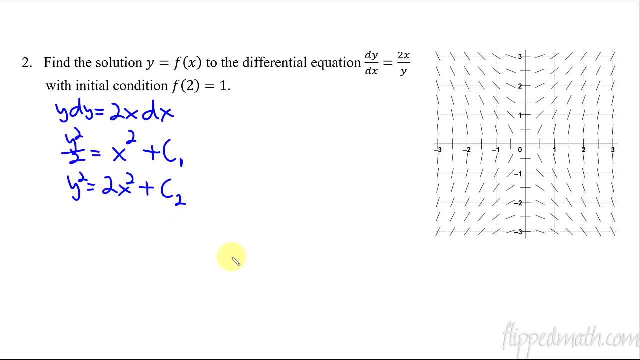 In here I'd end up with a 1 half, and then I got to work with fractions, And I'd rather not if I can help it. So now let's go ahead and figure out what this second constant is. So X is a 2, Y is a 1, so it's 1 squared. 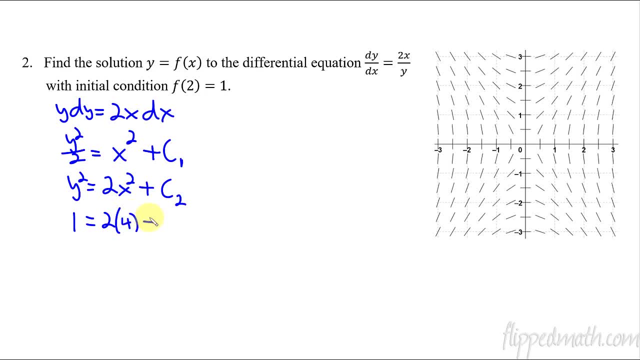 equals 2 times 2 squared is 4 Plus this second constant. So it's 1 minus 8. Negative 7 is what that little C 2 is. So let's take this line and start working with it now. So I've got y 2 or, excuse me, y squared. 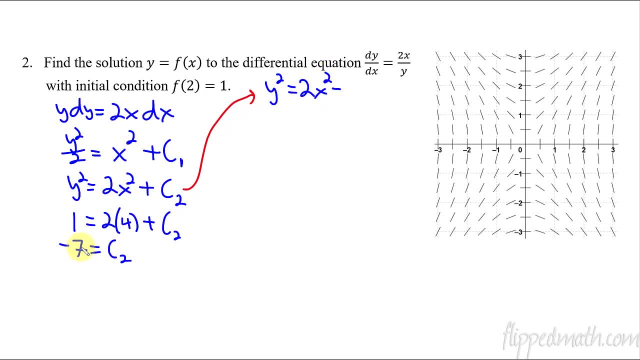 equals 2x squared plus my, Which was a minus 7, so minus 7. now I solve for y. Take the square root of both sides. when you take the square root you have a plus or minus. So I have the plus or minus the square root of 2x squared minus 7. 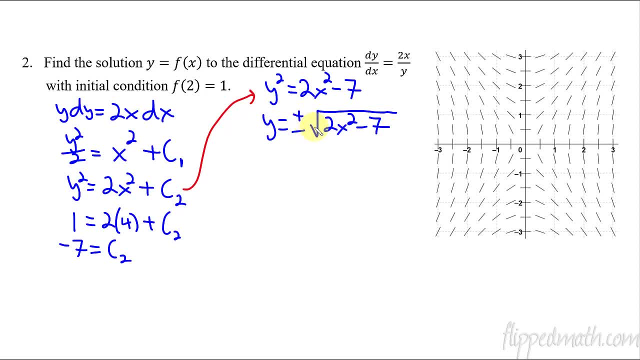 So the question is: is it y equals positive square root of 2x squared minus 7, or is it y equals Negative square root of 2x squared minus 7.. How do you know which one? we look at this point, It goes through the point 2, comma 1.. So let's go over here to 2: 1.. It's going through that point, right there. 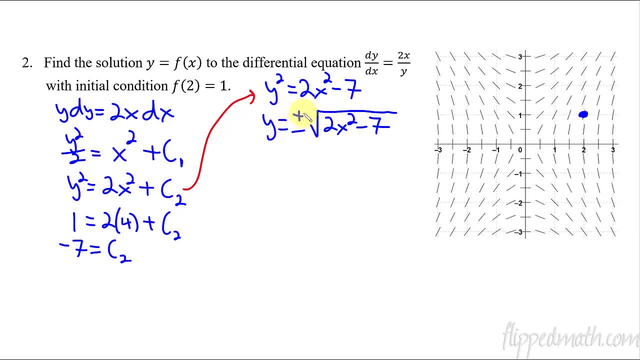 So y equals a positive number or y equals a negative number. 2 comma 1. that has to be positive. So I know it's not the negative square root, It is the positive square root of 2x squared minus 7.. So that is my answer. 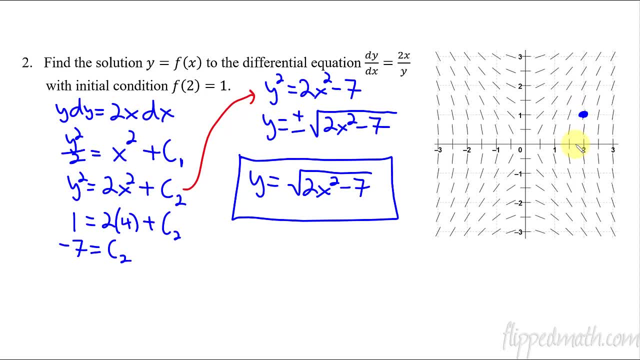 So let me show you what I'm talking about. the graph here then does something like this, And it kind of hands down a little bit there. That's what that graph is looking like. if I drew the other half of it, I could look at this one right here: y squared equals 2x squared minus 7. 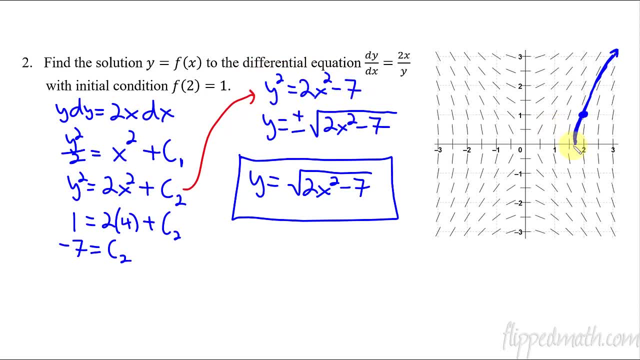 this is the implicit form of the equation and the graph of it is is a Hyperbola where it comes out like this and it goes off forever and ever. that's the graph of this one, But when you get the specific y equals equation, you only get half of it. You don't get both. 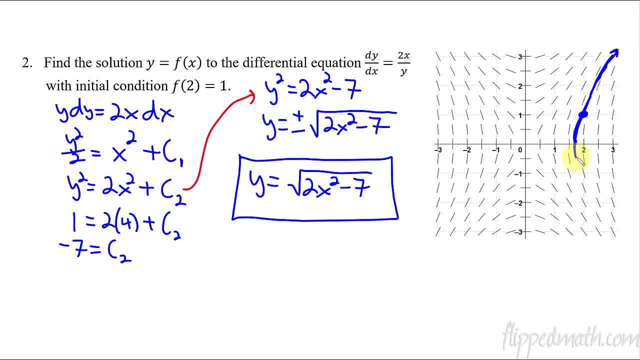 So that's why it is. the graph can help you understand which side- the top side or the bottom side- you're trying to graph. So when you solve it you'll have plus or minus And you have to think through with your coordinate point, which one was it? 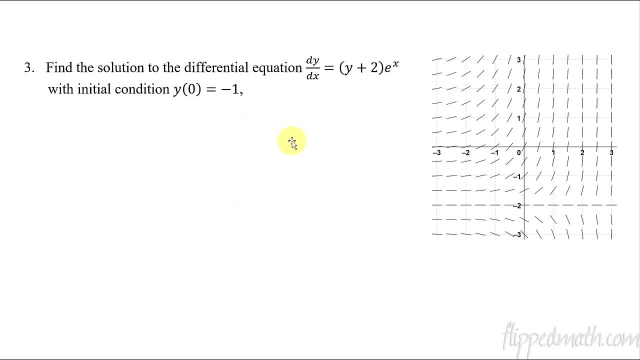 Okay, let's do one more example that's similar to that. So here we're gonna find a solution to the differential equation. blah blah, blah. All right, let's do it So. separate variables. I'm gonna divide both sides by y plus 2. 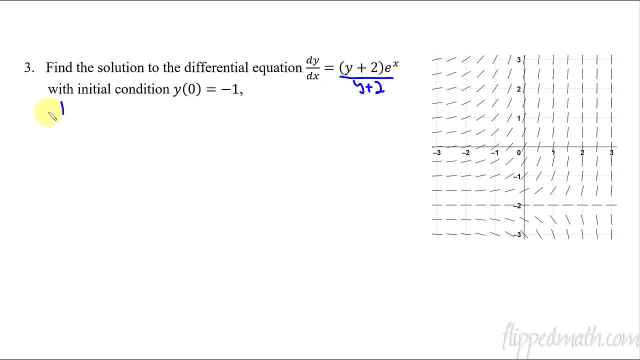 Y plus 2, y plus 2, so that gives me 1 over y plus 2, dy Equals. and then I have my e to the x dx. Now we integrate both sides. when you integrate both sides, you end up with the natural log of the absolute value of y. 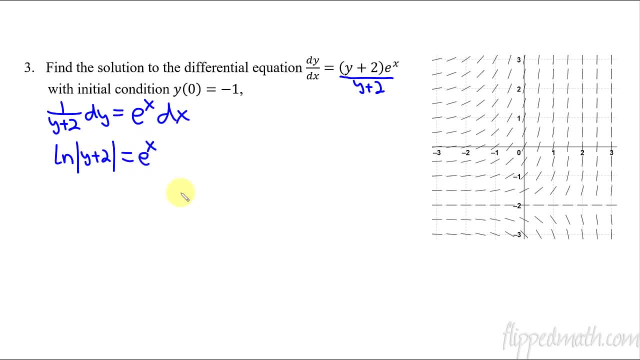 Plus 2, and that equals e to the x plus some constant. So let's see I could go Exponentiate both sides right, get rid of this, not natural log. But I think I, if I just plug in the negative 1 right now, I'm gonna do that. 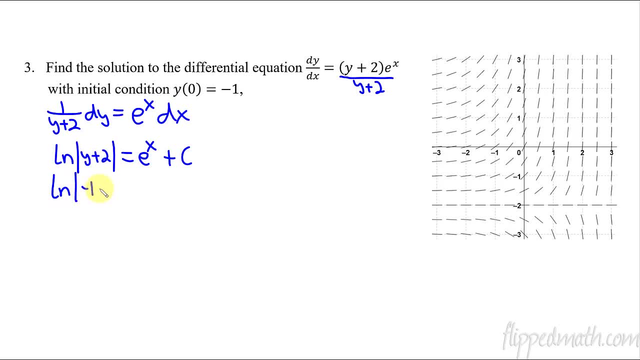 I'm gonna figure out what that constant is: natural log of Negative 1 plus 2. and then that equals e to the 0 plus a constant. So now that's natural log of 1 Equals 1 plus C. So natural log of 1 is 0. 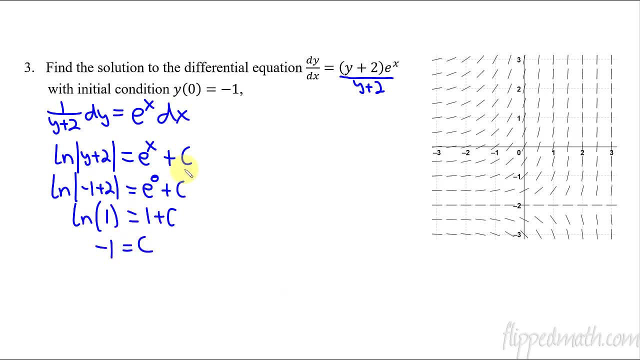 Subtract the 1, get negative. 1 equals C. Okay, all that just to get this little C here. So I'm going to start off. Let's rewrite this line. So I have the natural log of the absolute value of y plus 2 Equals e to the x minus 1, because that was my C. now we exponential exponentiate both sides. 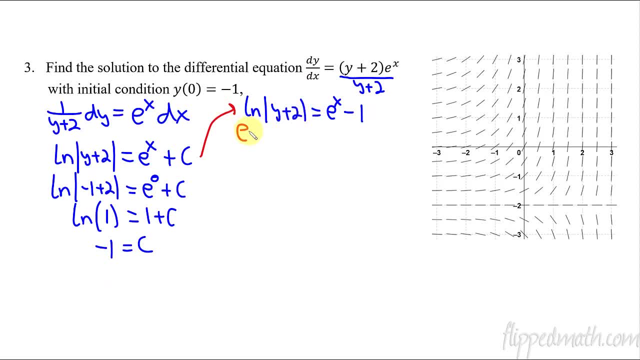 So I'm going to have remember exponentiate. We're gonna have e raised to that. e raised to that. It's gonna look weird. e to the e, So this is all gone. I have absolute value. of y plus 2 equals. this is weird. e raised to the e. raised to the x. 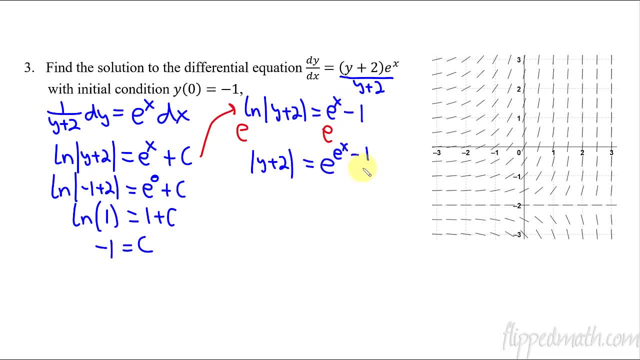 minus 1, so e raised to the x minus 1. now you could Put this together and make this e to the negative 1 in front. Alright, you could do that e to the negative 1 and just put this as an like it's coefficient, and that also equals 1 over. 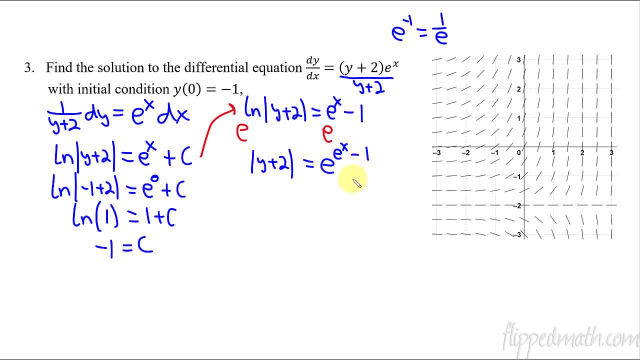 e, so it's up to you. I personally think this actually looks cleaner, But it just depends if it was a multiple-choice problem or not, Like how would they write it and you'd have to figure out to their equivalent. Okay, Now, this is the part I didn't really teach in the last lesson and I probably should have. I'm sorry when you get rid of. 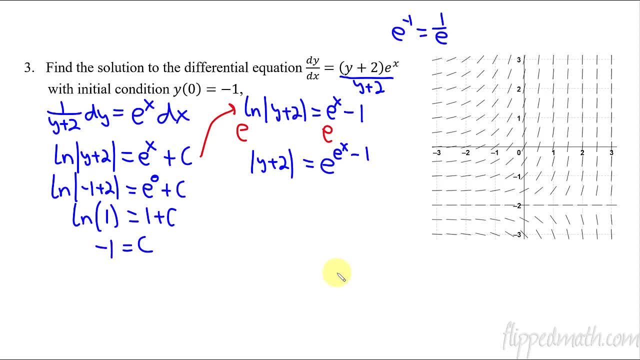 An absolute value. This is important because I didn't really cover this in the last lesson. when you get rid of this absolute value, You're going to have a plus or minus. Let me remind you something real quick, this problem right here. Remember back to our algebra one days, when you have to solve a problem like this in order to get rid of the absolute value. 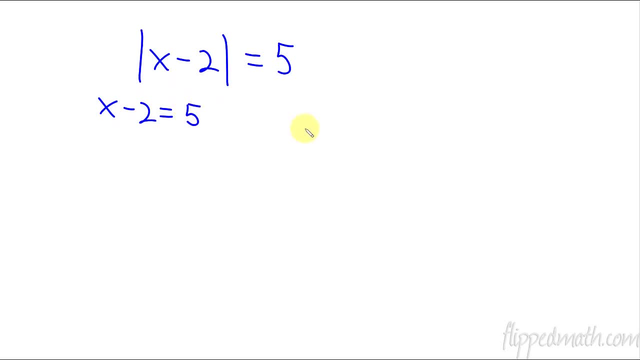 It actually becomes two different equations. It's x equals 5 or x minus 2 equals Negative 5, and then you solve both. you get x equals 8, If I knew how to add 7, and then on this one, x equals negative 3. now 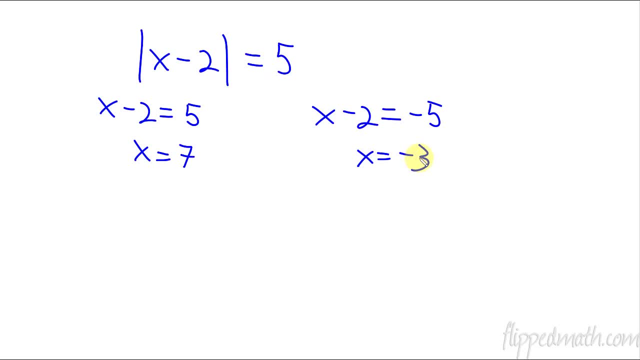 You see, the both of these work: 7 minus 2 is 5, and then negative, 3 minus 2 is negative 5. absolute values: 5. So when you get rid of the absolute value, the other side is a plus or a minus. so when I come over here to get rid of this absolute value, I'm going to write: y plus 2 equals a. 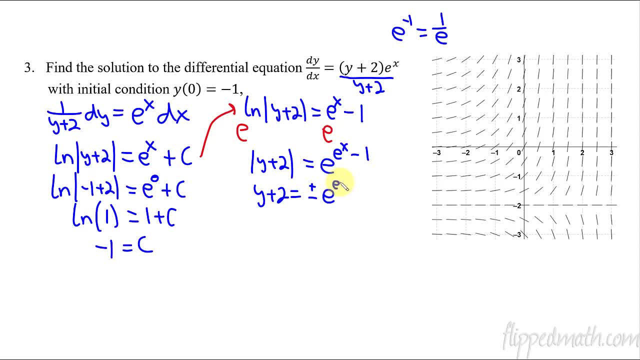 plus or minus e raised to The e to the x minus 1. So now I get y equals plus or minus e to the e to the x minus 1 and then subtract the 2 minus 2, So which one is it? Is it the positive or the negative? 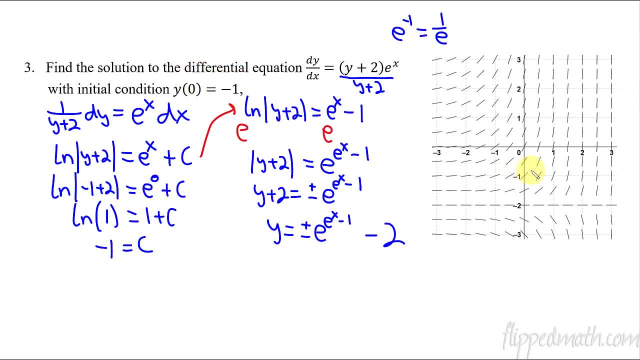 The initial thought is: well, look, here We have a negative y value. right, Where's 0 negative 1, 0 negative 1. We have a negative y value, So it must be the negative 1, but that's actually not true. 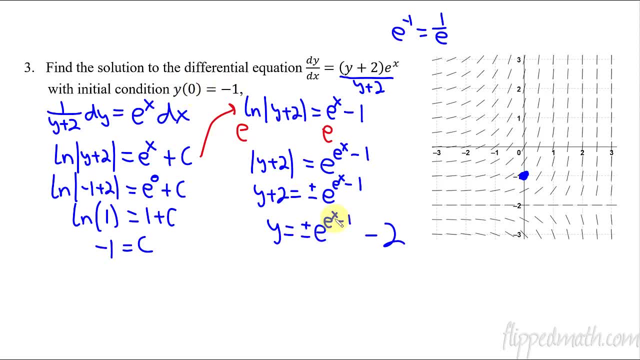 You have to try that. try the plug in the point 0 negative 1. if you plug in a 0 right here, I'm going to do this work on the side. So I'd have plus or minus e to the e to the 0, minus 1 minus 2. 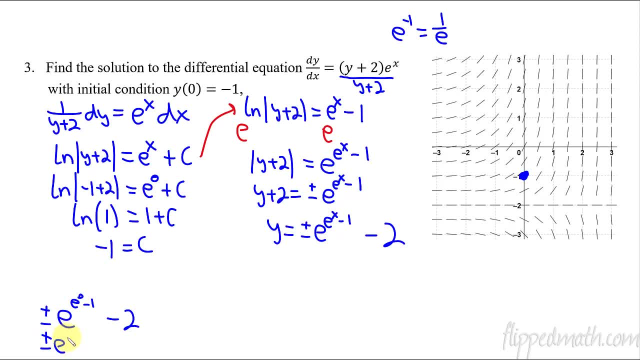 So then that's plus or minus e to the 1 minus 1 minus 2, And so that's just plus or minus e to the 0 minus 2. So this is plus or minus e to the 0 is 1 minus 2. 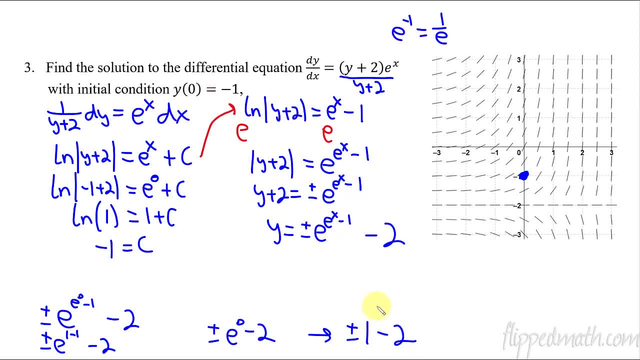 so which one makes this work? if I plug a 0 in which one of these gives me a negative 1- 1 minus 2- Or negative 1 minus 2, will it be the positive? so I want my answer to be only the positive answer. 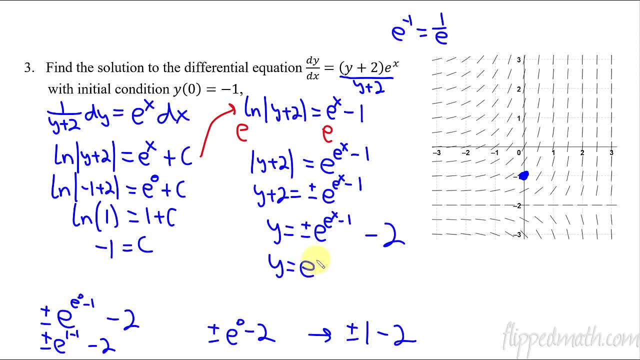 So my final is: y equals the positive e raised to the e to the x, minus 1, minus 2. That's the answer and you can see the reason why. if you look at this slope field- We've got our graph- that will come up and there is an asymptote here. 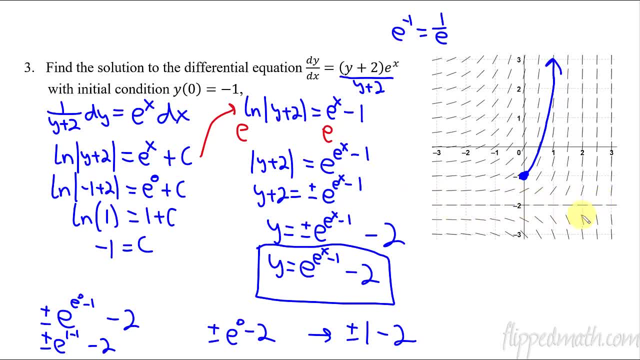 You can see this flat. if the y equals negative 2, you have an asymptote. So it's gonna approach like this: see, if it had been the negative, that would have been Down here on the negative side and it would be coming up. So yes, that is a bit tricky. but the slope field: this is where the slope fields kind of nice. 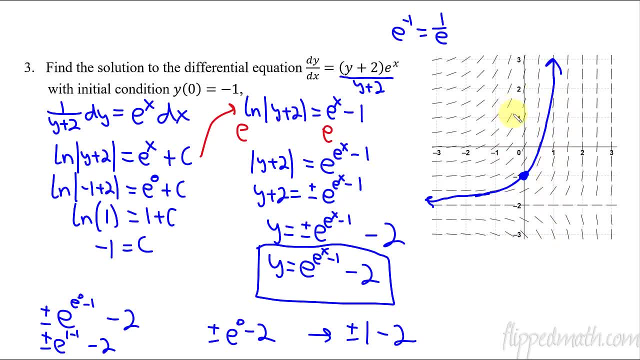 It can help you when you sketch the graph to kind of get an idea: Is it the above it, Is it below it? Okay, so I tried to give you in this lesson- I actually gave you some of the more challenging ones So that you didn't freak out when you see some of these other problems. 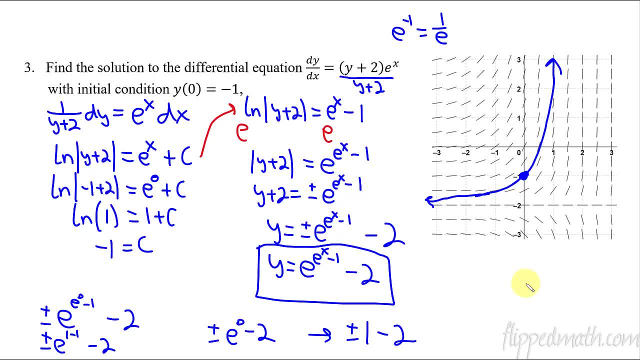 So a lot of the problems will be easier than what I just showed you in this practice, Although your test prep. you're gonna have us a little bit more test prep on this one. We didn't have a test prep in the last lesson, So this one will have some more. 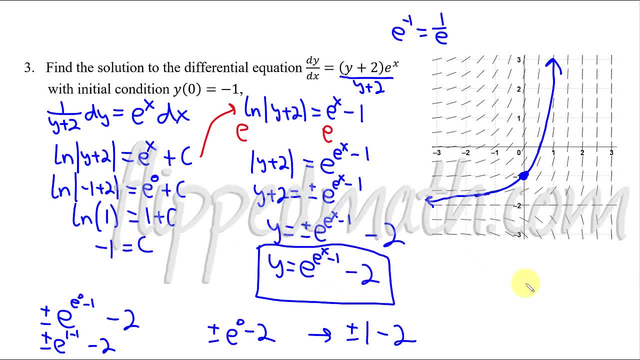 So rock that master check. We Don't finish with this and I'll see you back in our next lesson.